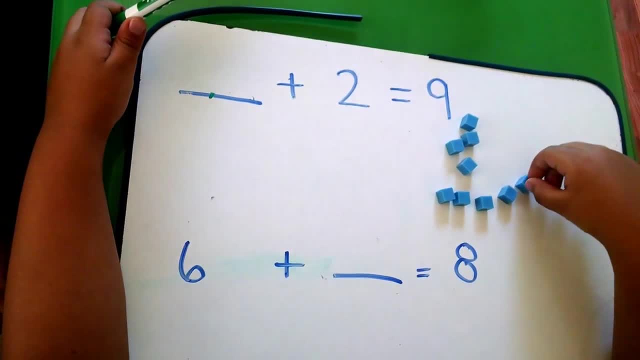 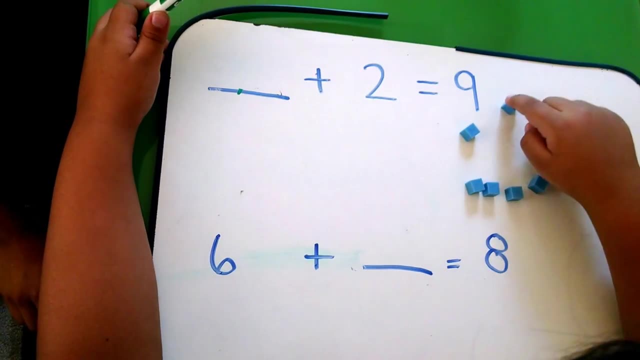 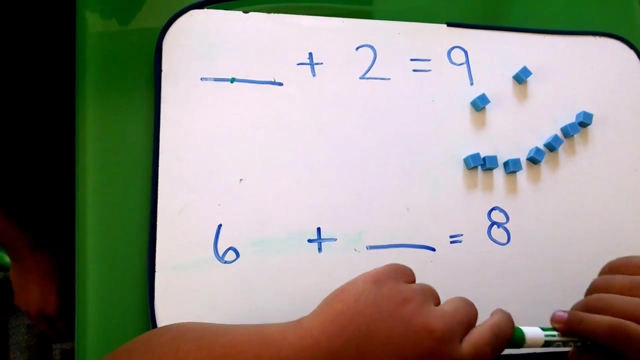 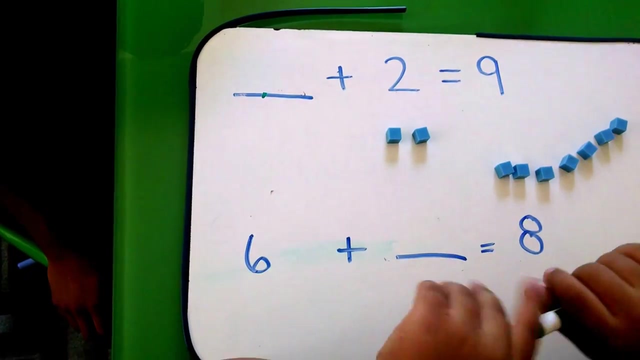 And put them in order like a line. You can drag them there if you want. Okay, so you got the nine blocks. Take away the two blocks And then put it under the two And then take the rest of the blocks. 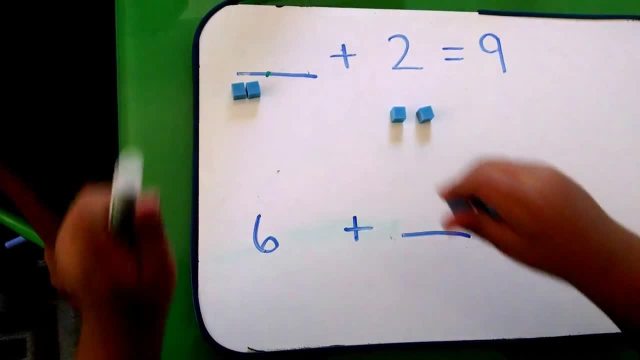 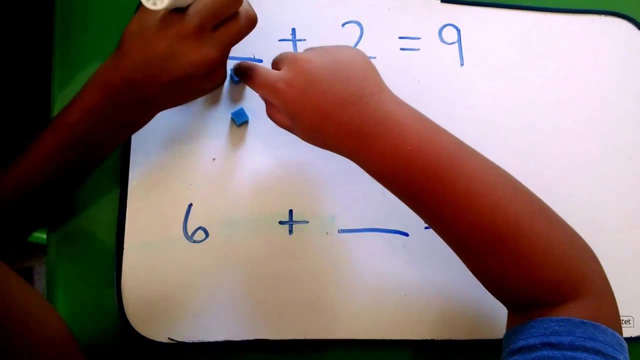 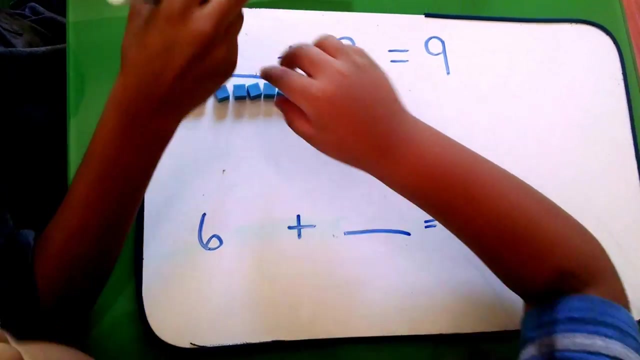 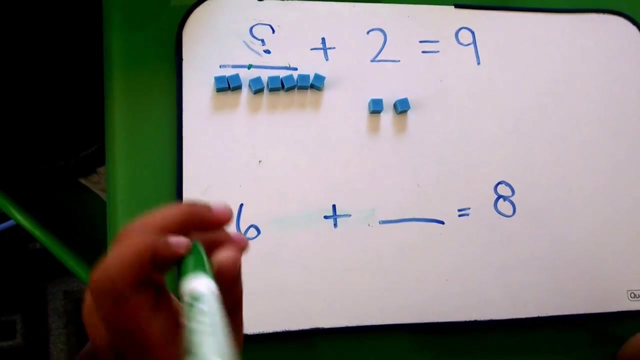 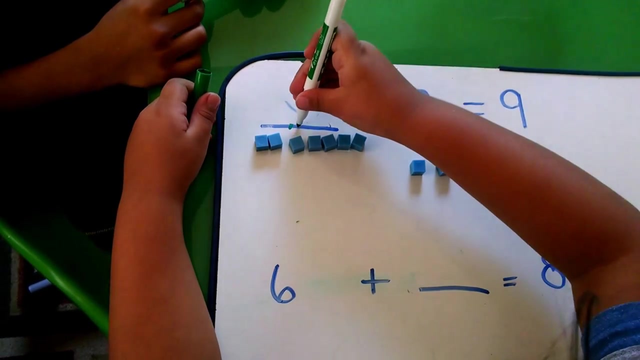 And put it under the what sign. So there's seven blocks. So that's the answer. So you have to take away the what sign And then you have to write seven, Because that's the answer. That's not how you write seven. 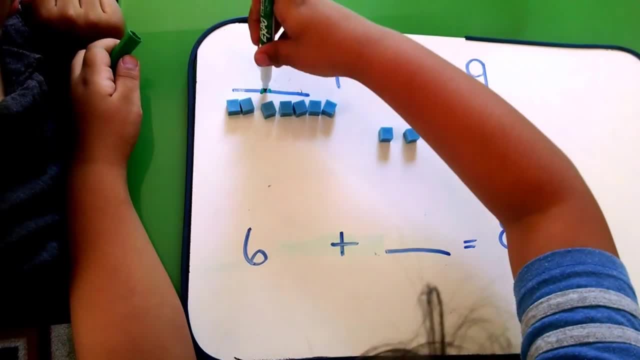 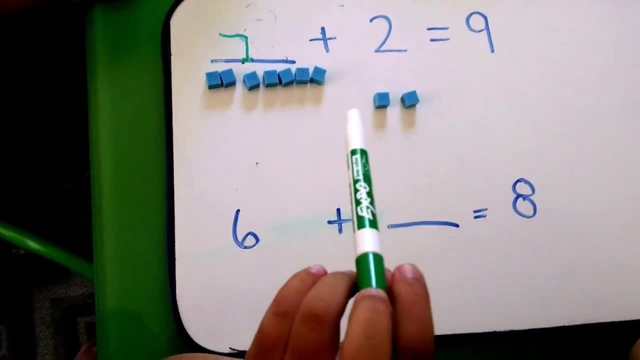 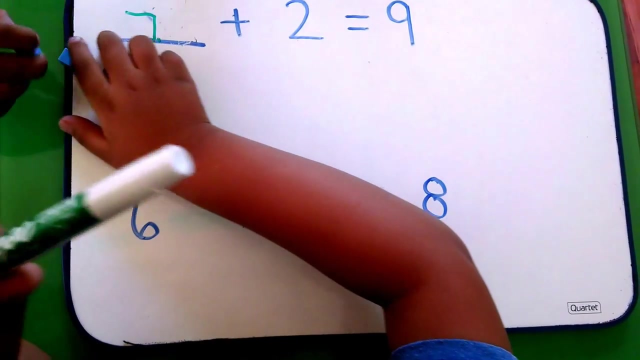 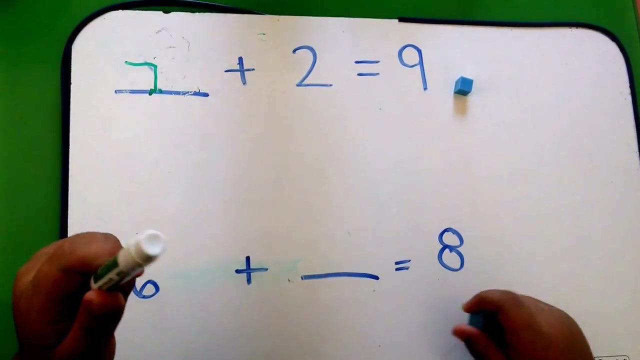 Okay, Okay, And then the next. the second round is kind of easy. So you're going to take away the blocks from the nine, Put one next to the nine, because you'll need that one. So you put one, This one, I got one. 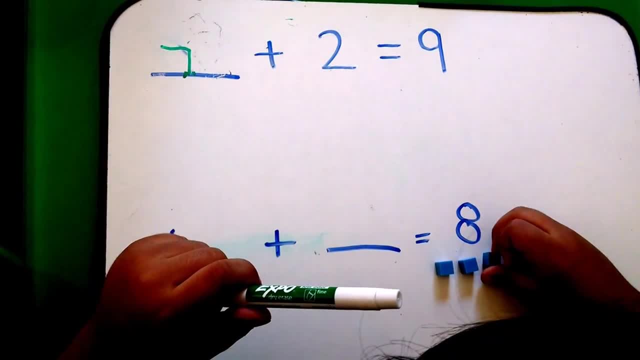 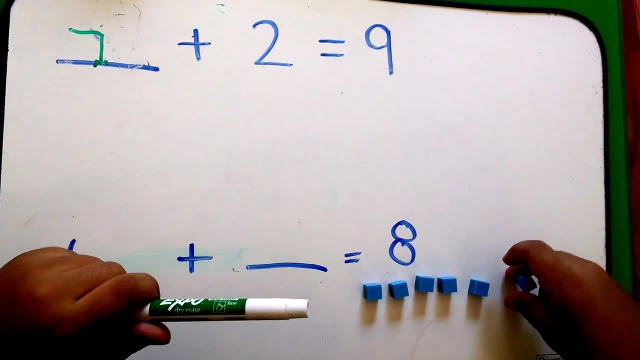 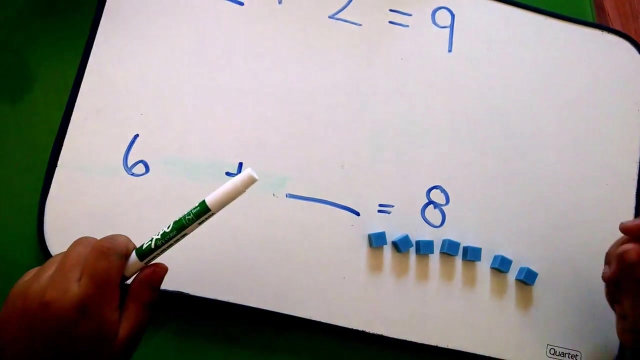 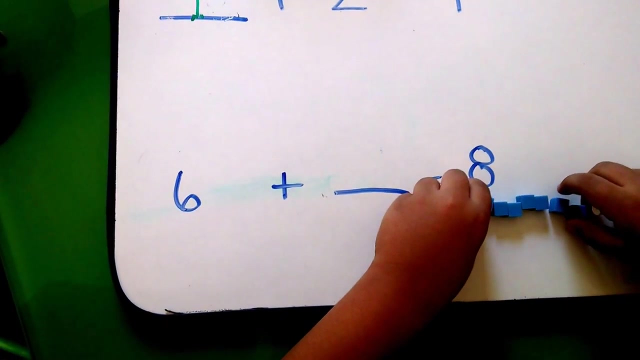 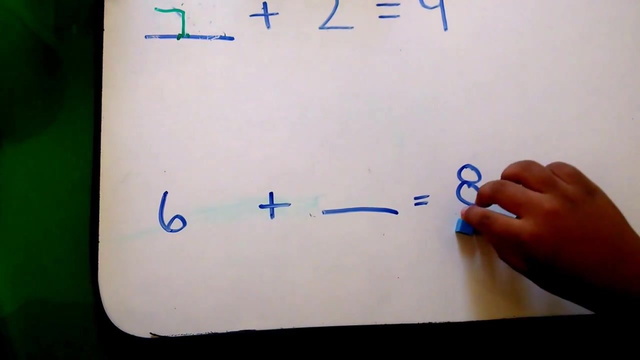 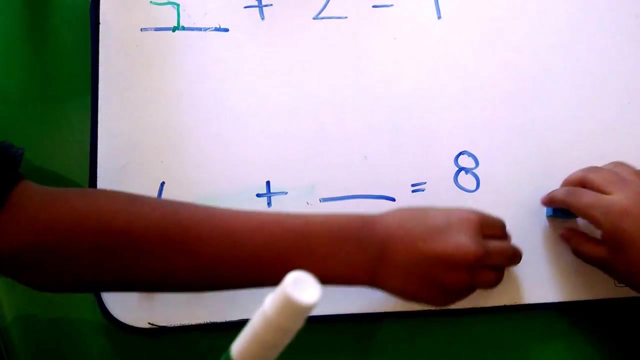 So you put one, two, three, four, Four, five, six, seven, eight There. Now you take away six blocks: One, two. One, two, three, four, five. That's it, That's it. 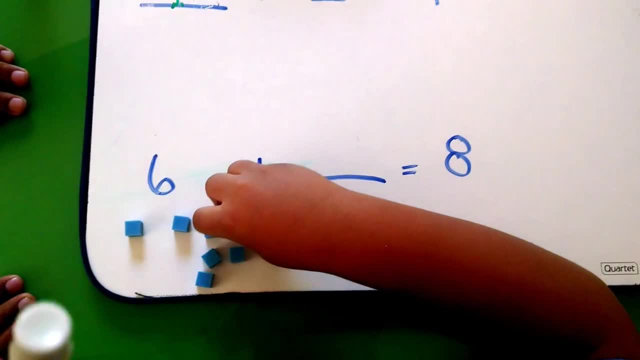 Five, Six, So six blocks, Jack, what are you doing? One, two, three, four, five. Take them. Wait, Yeah, You're missing me. Oh, Mom, Can you start the video over again? It's okay, Just go. 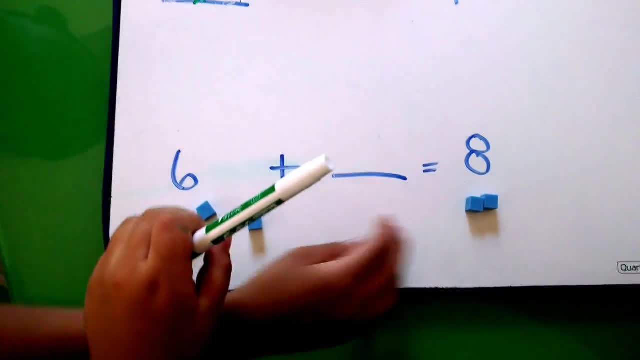 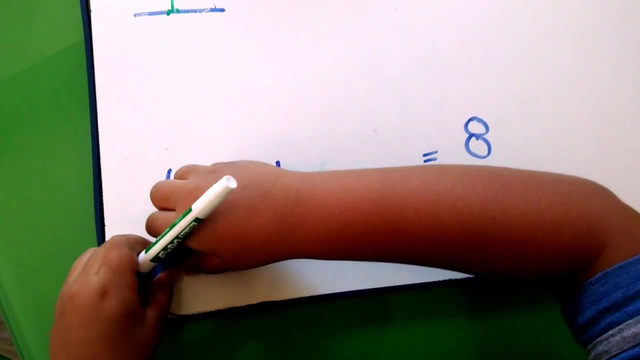 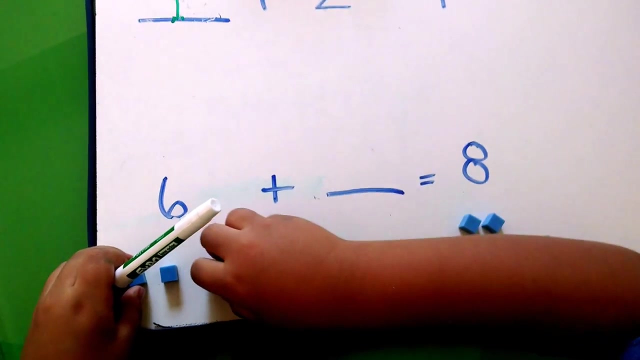